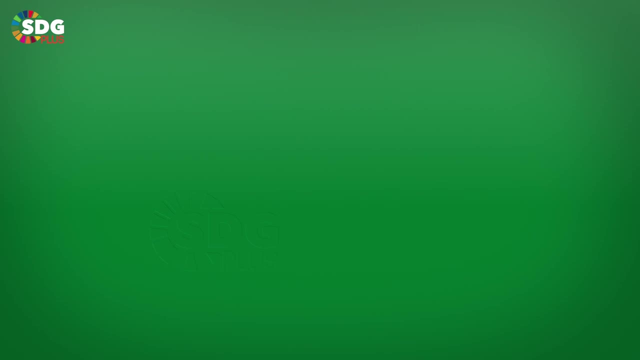 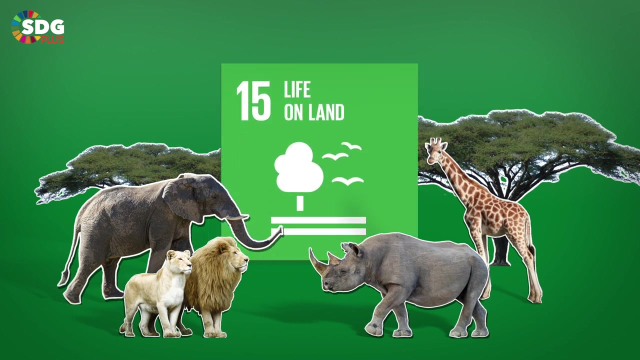 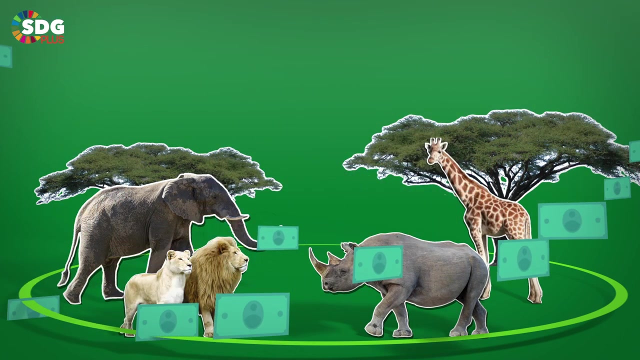 wildlife conservation in Kenya. The aim here was to save endangered animals and make progress in achieving SDG 15 – Life on Land. Over the past few decades, rich countries have made significant contribution towards wildlife conservation in Kenya. This meant wildlife reserves became bigger. 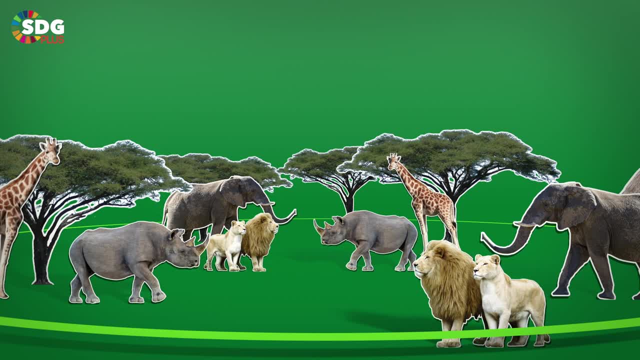 and the animals were no longer endangered. However, this expansion came at a cost. The growing wildlife conservation in Kenya is an important part of the development of wildlife conservation. The growing wildlife conservation in Kenya is an important part of the development of wildlife conservation. 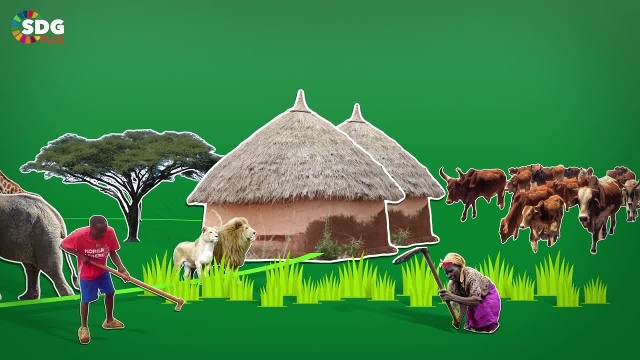 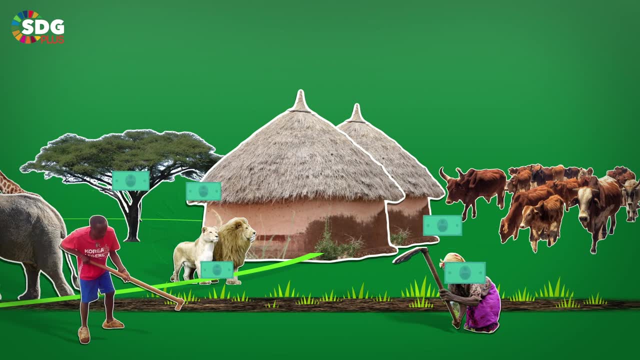 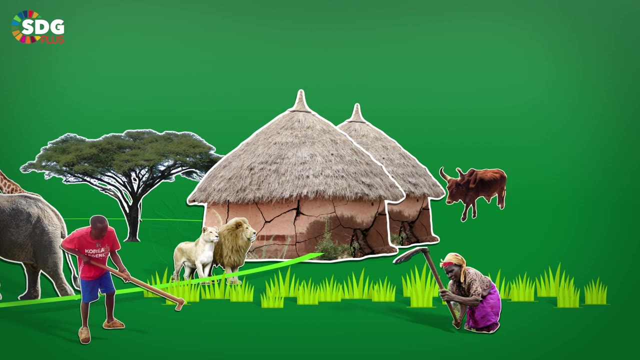 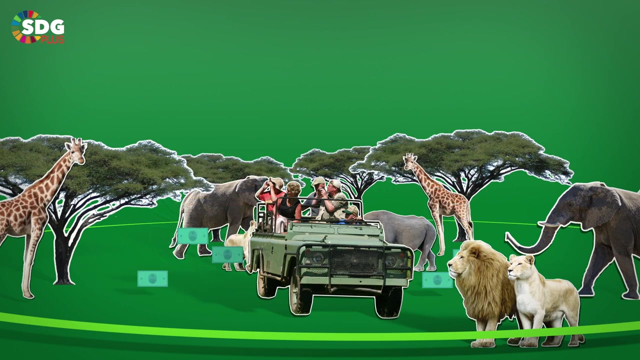 As the wildlife population started to encroach neighbouring communities' lands. these wild animals would often invade and damage local farmlands. To restore the lands, the poor farmers were often found paying from their own pockets. This gave rise to high levels of poverty in these areas. The big wildlife reserves did attract rich tourists. 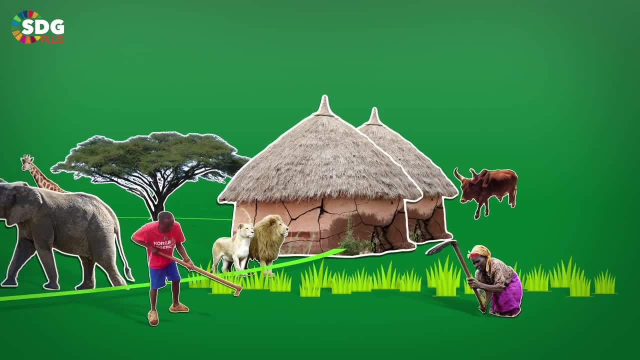 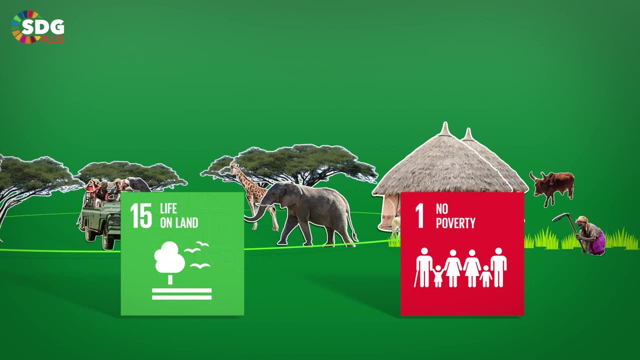 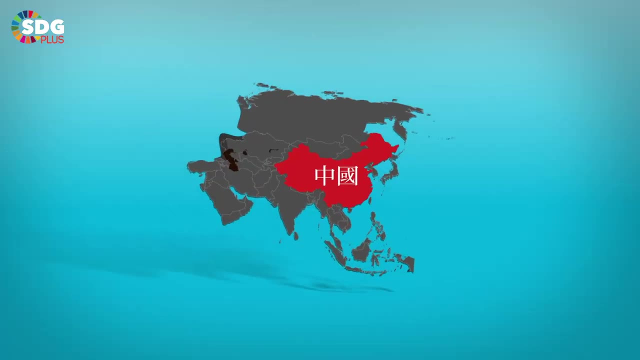 But the tourism money rarely trickled down to these communities In other. In other words, trying to achieve SDG 15 made it more difficult to eradicate poverty. Favouring the environmental pillar meant overlooking the social pillar. On the other hand, one of China's primary focus has been to drive economic growth started. 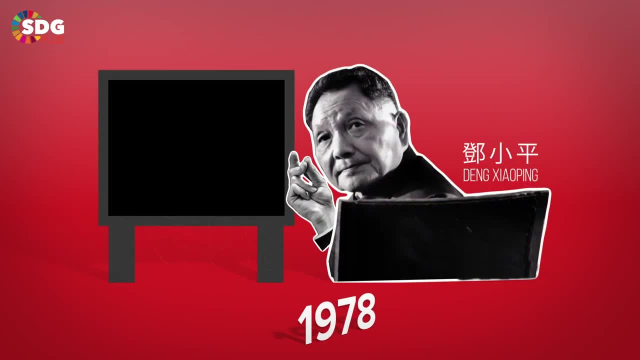 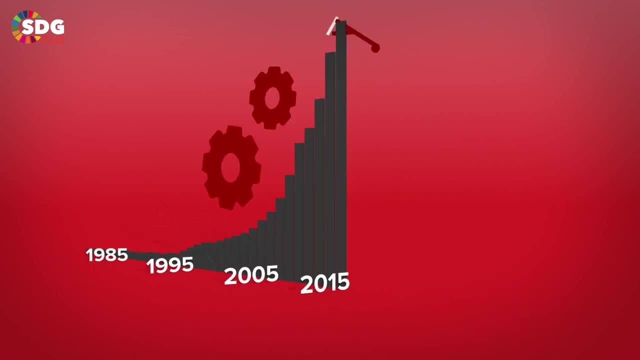 with a reform in 1978 that opened China's market to the world. Since then, China has been enjoying an explosive GDP growth. This has helped lift 850 million people out of poverty, with only 3% of China's population currently below the poverty line. 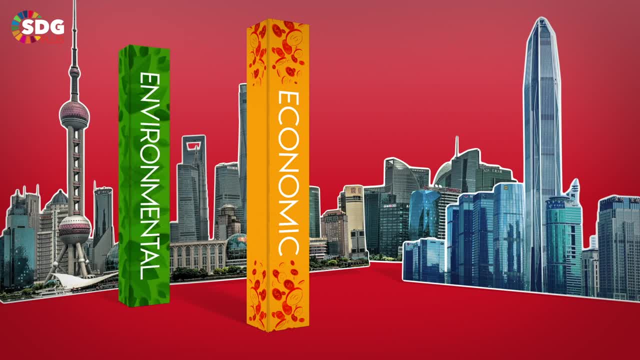 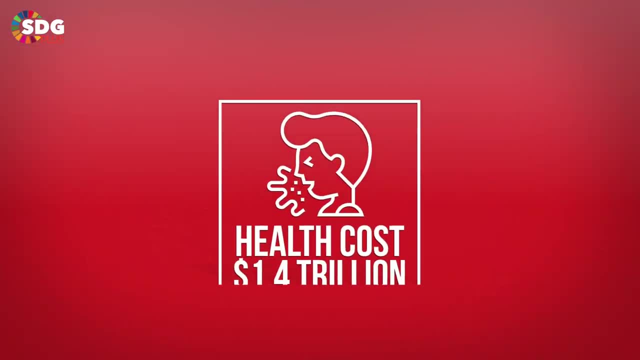 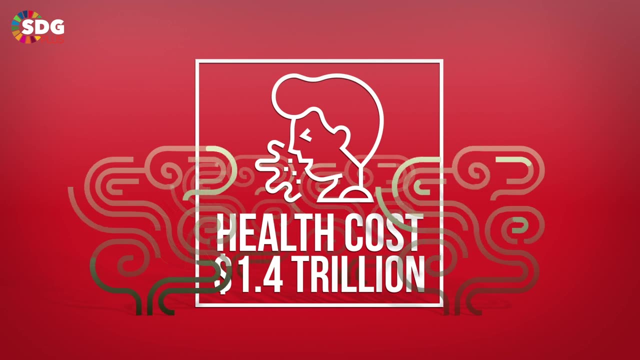 During this period of economic prosperity, China's environmental and social pillars took a hit. A 2017 report estimated that China will suffer a health cost of $1.4 trillion because of its air pollution. On top of this, China's geological survey showed that the population of China has grown. 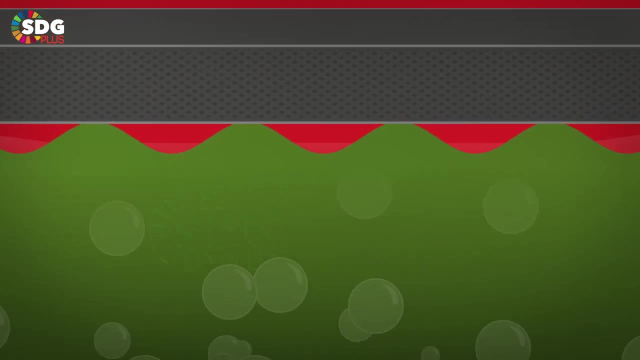 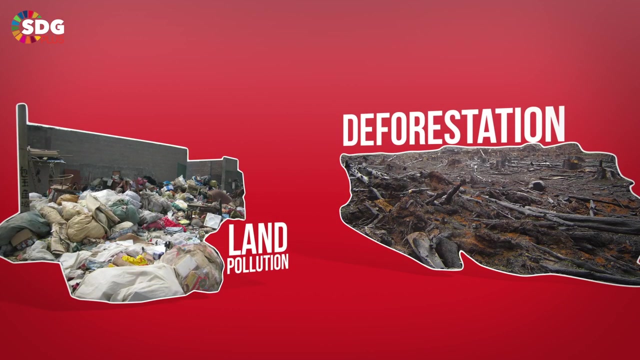 more than 1.5 times the size of the world's average population, which is about 1.5 times the size of the world's average population. The survey reported that nearly 90% of Chinese cities had polluted groundwater. Simultaneously, China is also dealing with land pollution, deforestation and poor animal.